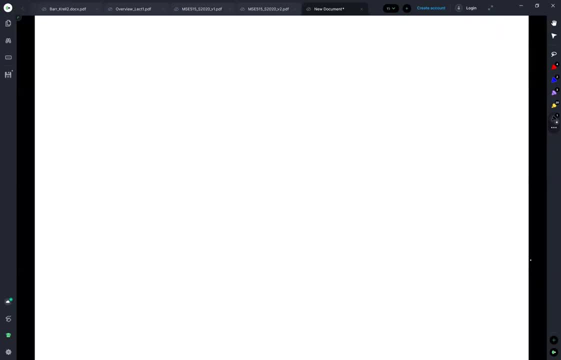 I thought I'd begin this presentation by deriving the triple product rule. I showed the triple product rule in lecture but didn't show where it came from. So the triple product rule starts out with some function of three variables, which we're going to call x, y and z, and it being equal to zero. 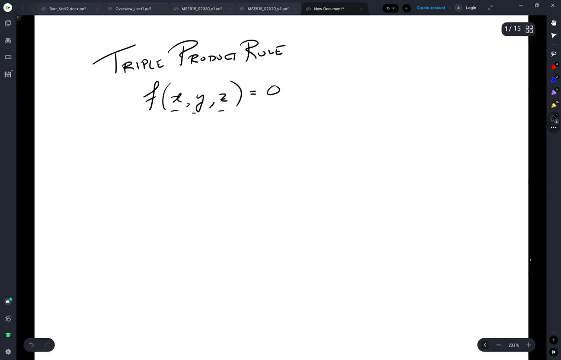 Now, each of these variables we can write out as a total differential, But we're only going to need two of them, So we'll write the differential in terms of x, x plus y, dy by dz, dz. Okay, so we've got these two differentials. 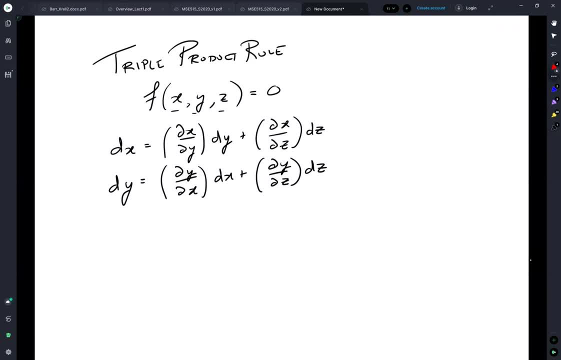 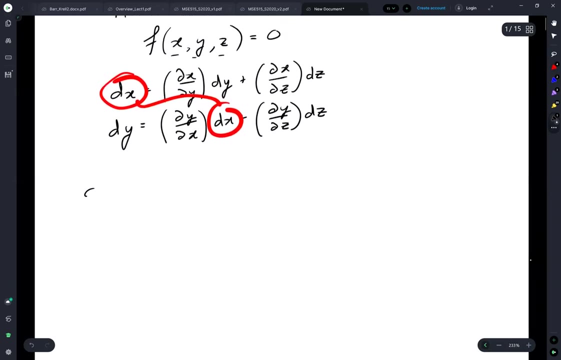 And now we're going to take and we're going to substitute dx into dx. That's going to give us dy is equal to dxdx by dx, which is, oops, sorry, partial With respect, I'm going to erase that. 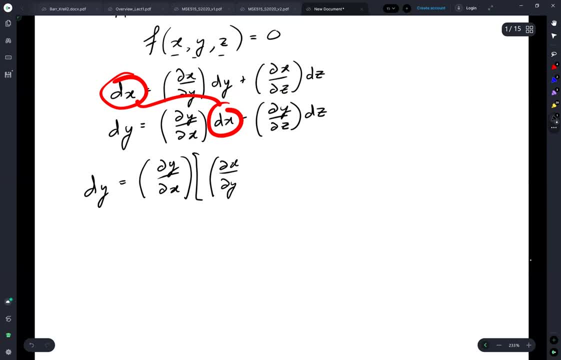 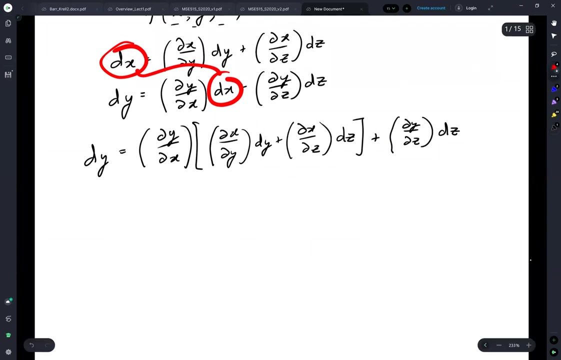 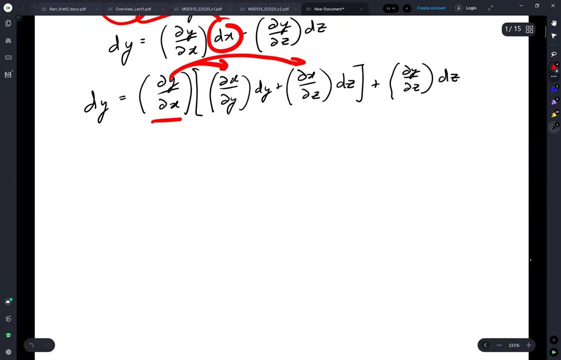 Partial with respect to x. Sorry, y of dy plus dx, dz. clues, It's not Quadrat d, z plus our term on the right, dy by d z, d z. Okay now, taking and distributing our dy by dx we get dy is equal to dy by dx. 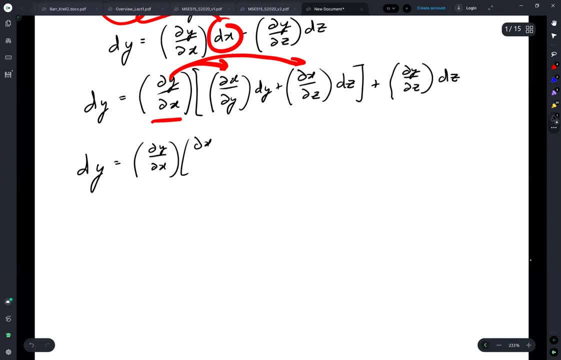 dx dx by dy dy plus dy by dx, dx by dz dz plus dy by dx dy by d z d z. Okay, great, Now this term here we got a dy by dy dx dx. 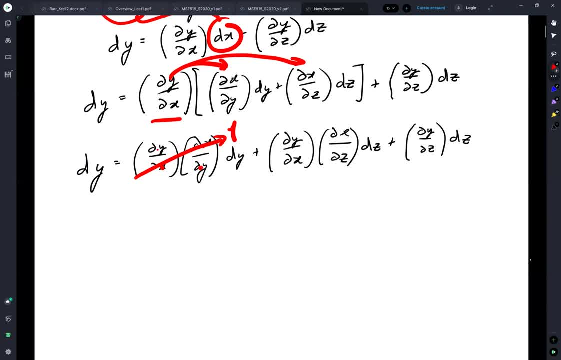 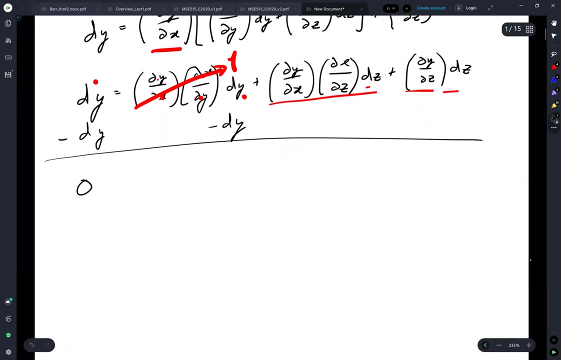 That's just one. So now we've got a. dy is equal to dy plus this term, plus this term, These dzs are going to get collected. But, Most important, we want to get rid of this dy. So we're going to subtract dy from both sides, which is going to give us 0 is equal to. 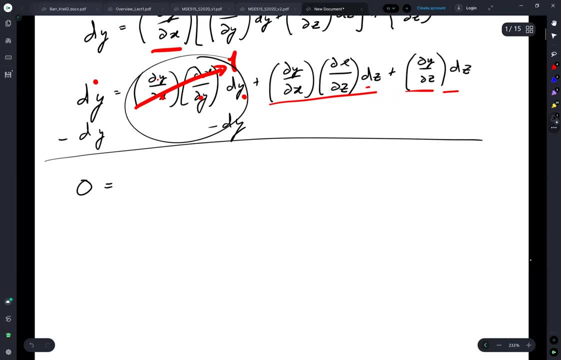 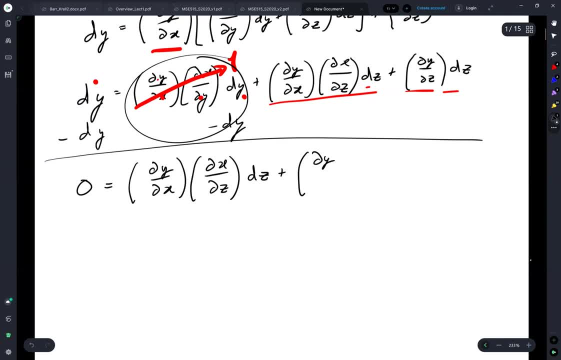 dx plus dy by dz, dz, And this is starting to look a little closer to what we're expecting, right? So we take and we multiply both sides by 1 over dz. So multiplying 0 by dz goes to 0.. 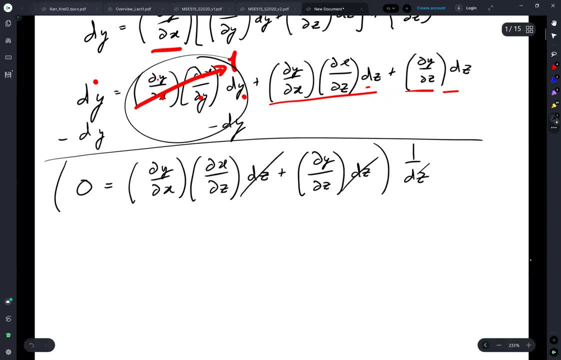 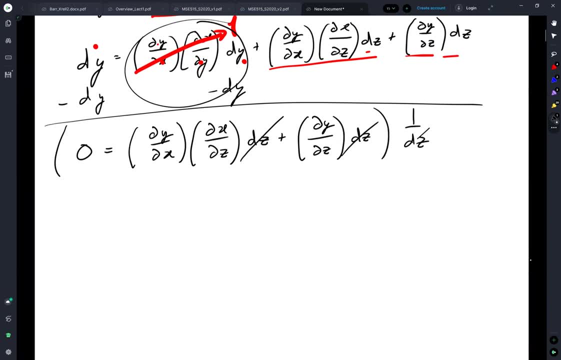 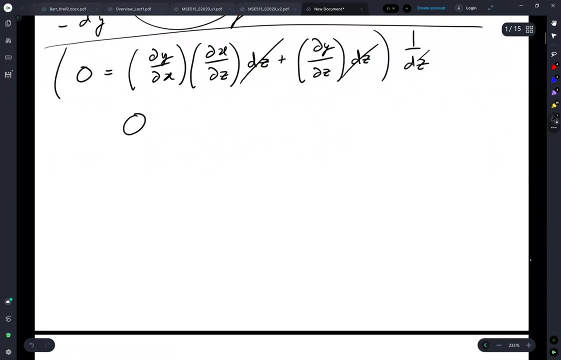 And on this side they're going to cancel, And on this side they're going to cancel, And on this side they're going to cancel And we're gonna wind up with 0.. Whoops, whoops, And we'll wind up with 0, which equals dy by dx, dx by dz plus dy by dz, or x by dx by. 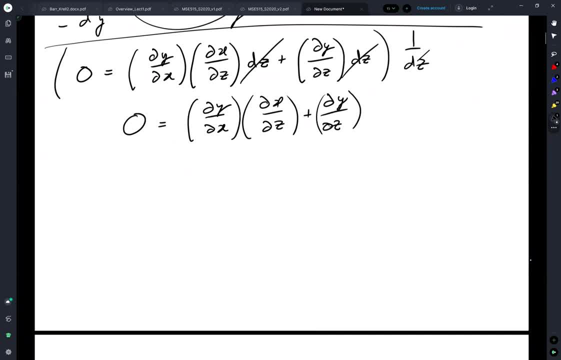 dx or y by dx, Like we said, y by x and y, Like you said, y by y, Which is just like nothing. It doesn't matter, It's just like nothing. We subtract dy by dz from both sides. 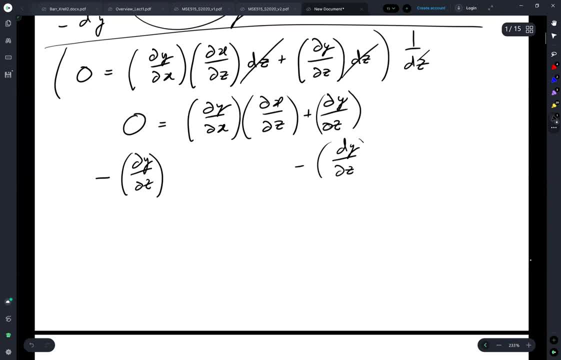 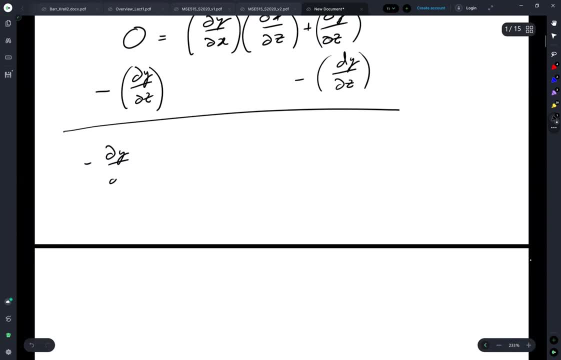 giving us minus dy by dz is equal to dy by dx, dx by dz. Now multiply both sides by dz by dy, So now on our left side we have dy, dy, dz, dz. So that's going to be 1.. 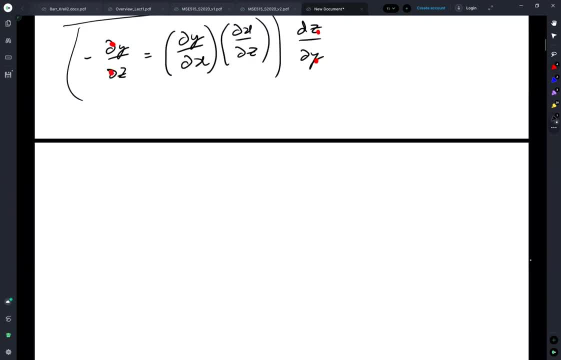 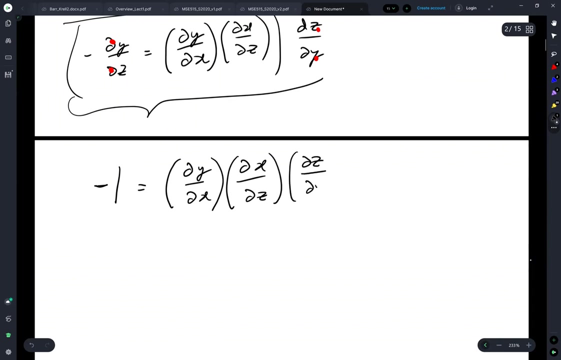 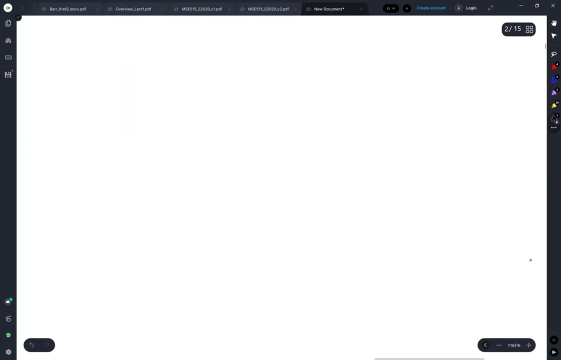 And this entire term now becomes 1 minus is equal to dy by dx, dx by dz, And this is the triple product rule that I showed during lecture, And I don't know if there's a way to generalize this. I don't think that there is. 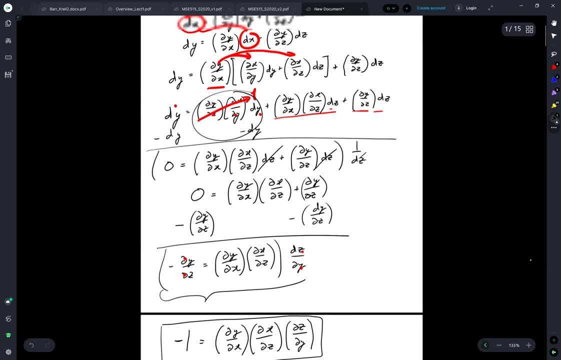 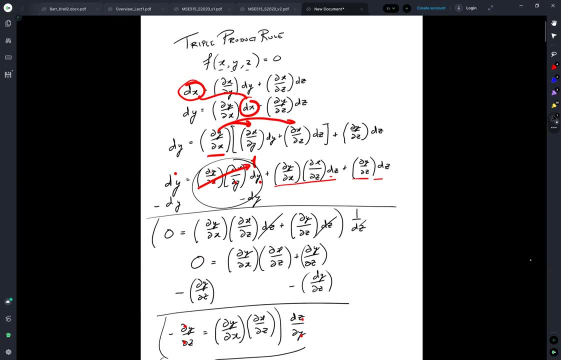 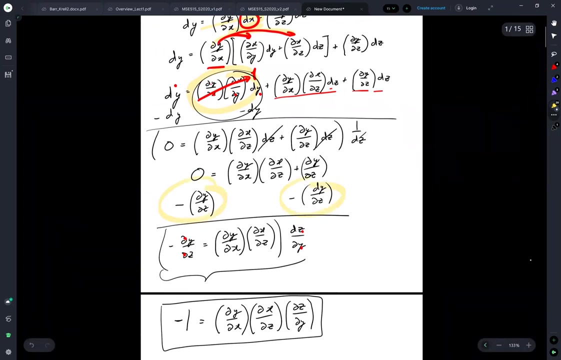 But nonetheless, the important thing is the basic math tricks that I'm showing here. you should be familiar with the ideas of substituting, Substituting differentials into each other, distributing, having cancellation, And then you know the ever popular trick of adding and subtracting to the same sides. 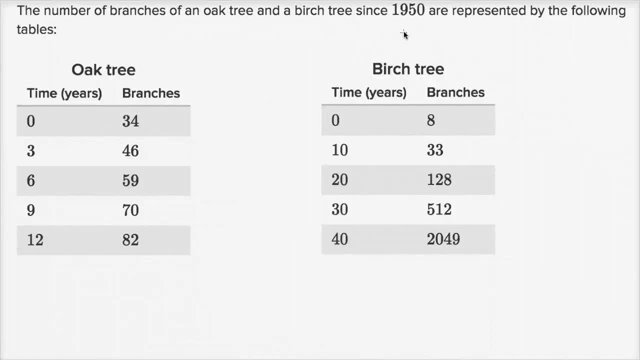 The number of branches of an oak tree and a birch tree since 1950 are represented by the following tables. So for the oak tree, we see when time equals zero has 34 branches. after three years it has 46 branches, so on and so forth. 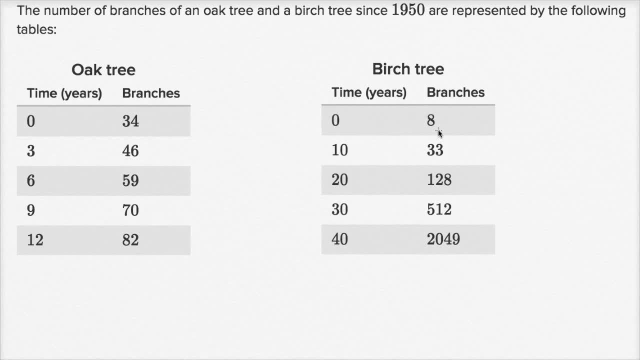 And the birch tree- they give us similar data at the beginning- has eight branches. in 10 years has 33 branches, and they give us all of that. And what I wanna think about in this video is how should we model these? 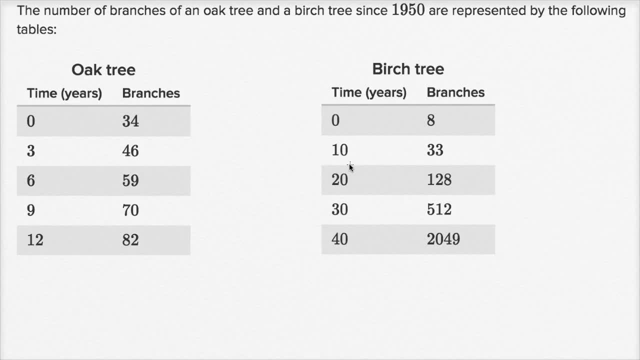 So if we wanna model these with functions and the choices we'll give ourselves, there are other options. but the choices we'll give ourselves in this video are linear, and linear versus exponential functions. Which of these are going to be better for modeling? 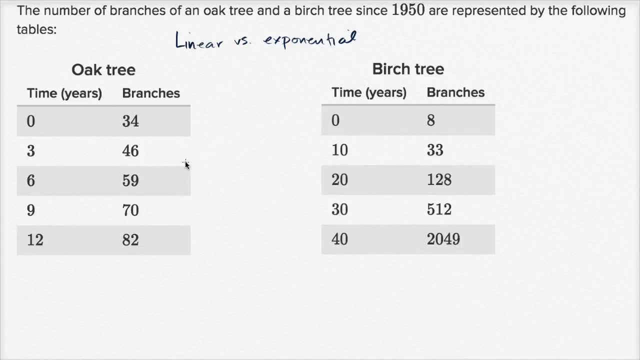 for modeling these, this data. So let's first look at the oak tree, And the key to realization is whenever I have a fixed increase in time. so each of these steps, this is plus three years, so it's a fixed increase in time. what happens to my number of branches? 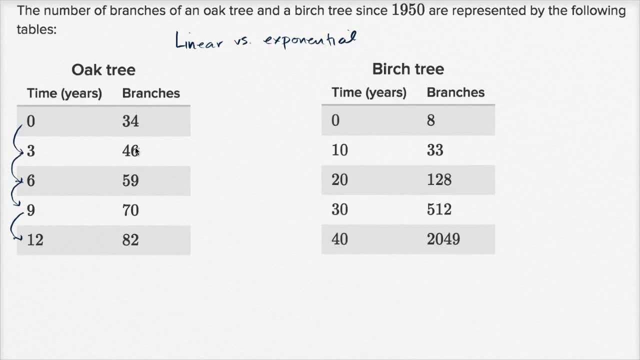 Is it going to be a fixed change, in which- or roughly a fixed change, in which case a linear model might be good, Or is it going to be a change that's dependent on where we were? So what am I talking about? 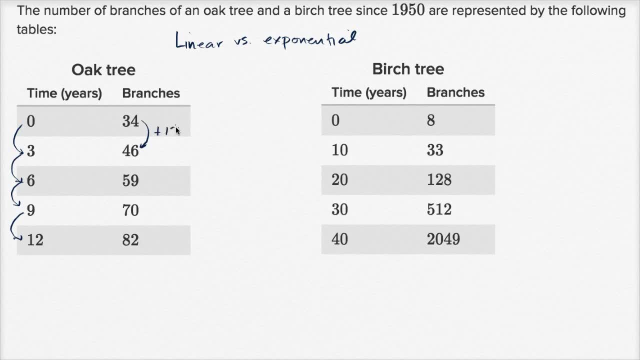 So 34 to 46, that is plus 12.. 46 to 59 is plus 13.. 59 to 70 is plus 11.. 70 to 82 is plus 12.. And so this isn't an exactly fixed change.